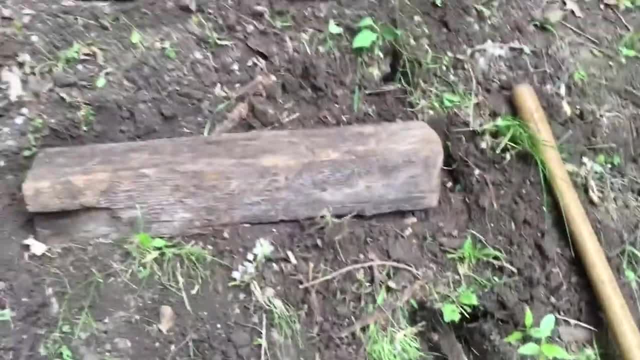 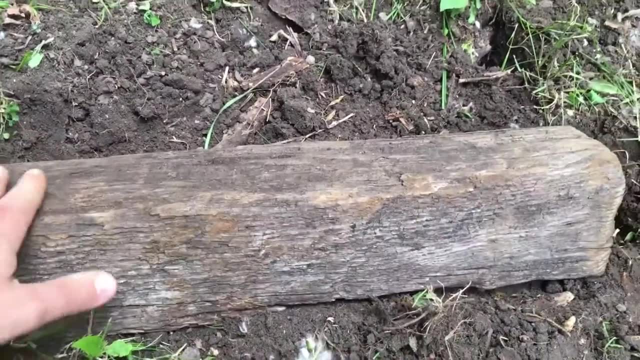 tall From then. once you have it set, you can set it, level it with a level. You want your steps to be angled up the hill a little bit, so it'll be level this way and then tilted it back this way. 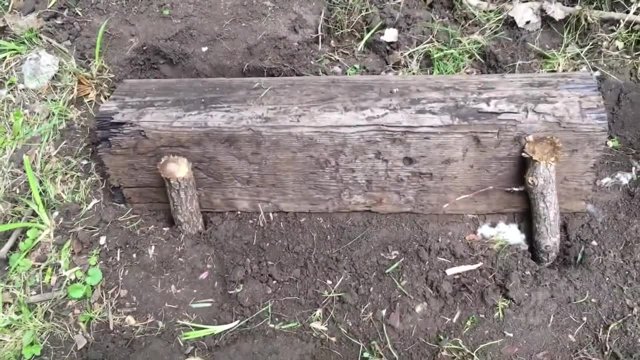 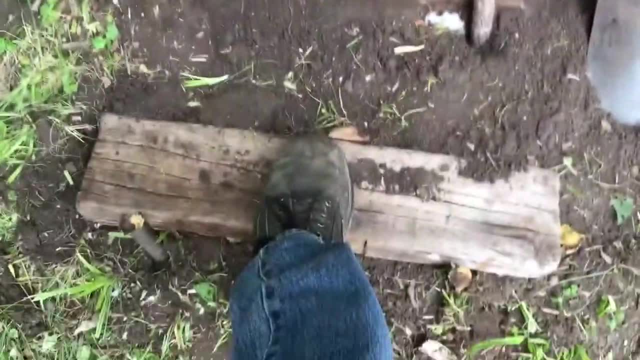 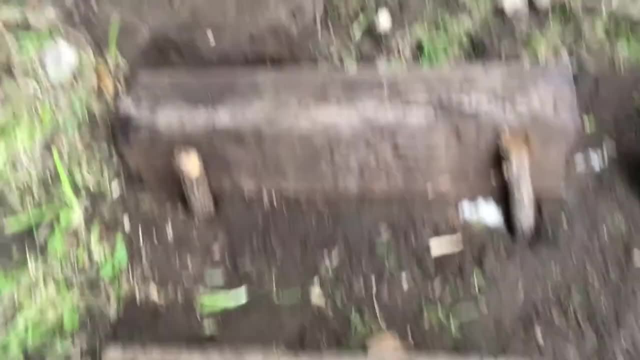 Then you can use either stakes or rebar. If you have short steps, you probably want to use stakes, because there isn't a lot of room for a foot. So if you put rebar in there, someone could step on it and maybe injure themselves. So you can put some stakes. Now you can either buy stakes. 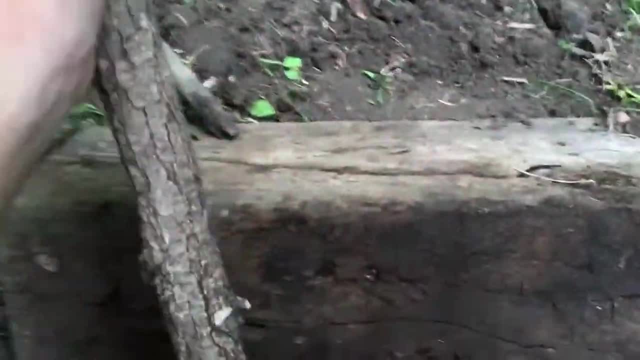 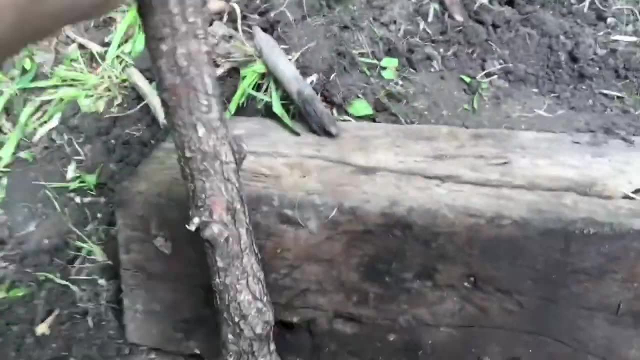 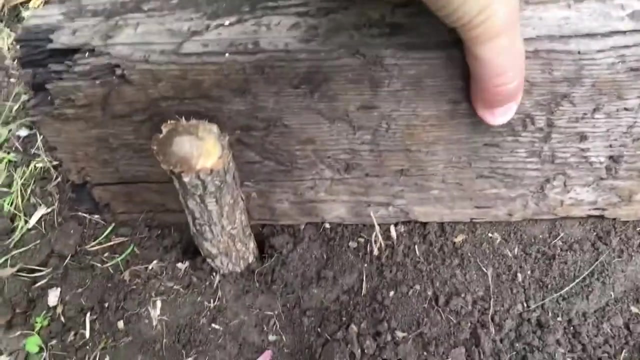 or cut them yourself. If you cut them yourself, make sure you use a strong, hard wood. Something like ironwood works very well, And then you can set it right like this and pound it in. As you can see here, I've got one pounded in already. It makes the step a lot more solid. And then here: 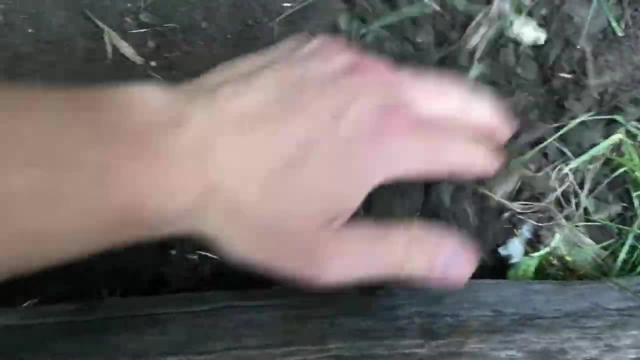 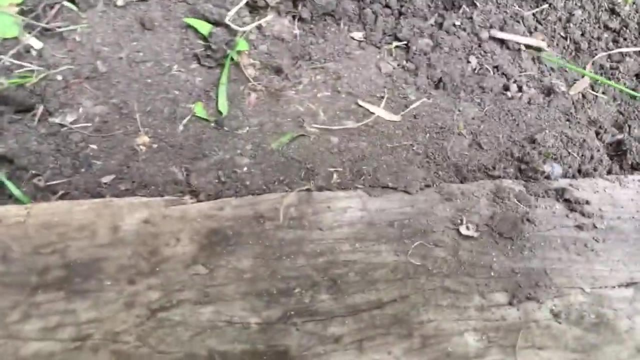 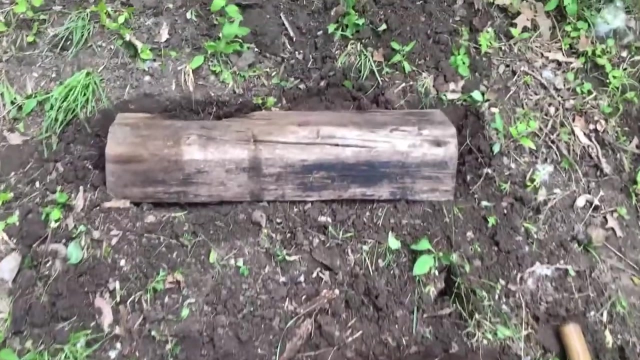 you'll want to pack dirt around the step. So you have that packed in, get some water so it settles and is solid and looks more like this. So that means there will be some really solid steps. So, as you can see, I've got the groundwork laid For all of these. I've got them in and they're. 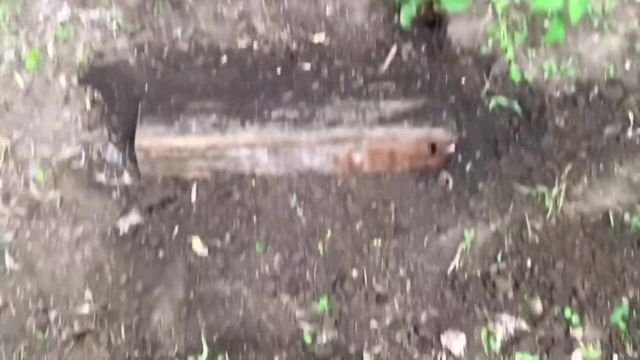 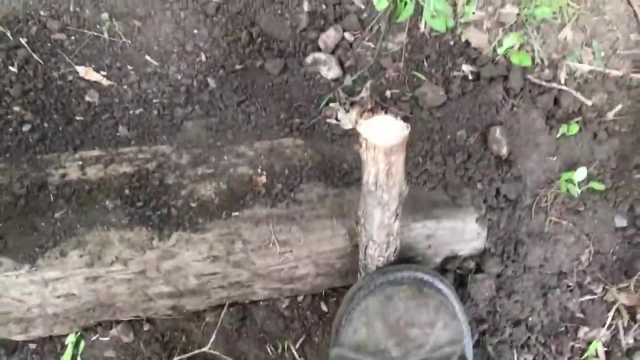 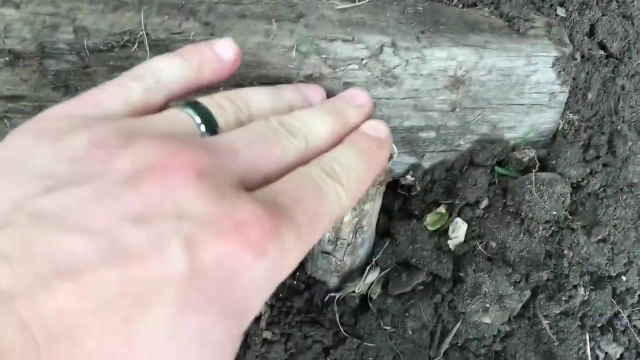 ready to be staked. So I'll show you what the finished product looks like after staking them in. There you go. You want to sink the stake a little below the step so that someone doesn't step on it or stub their toe. 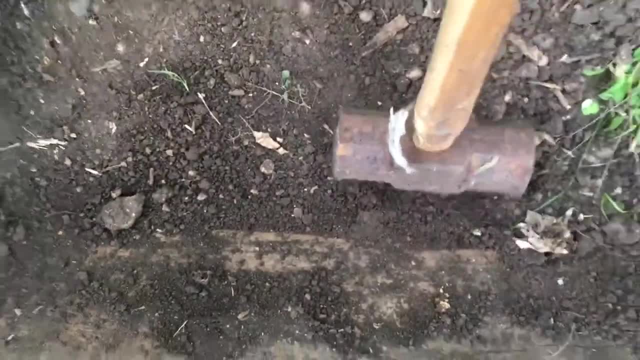 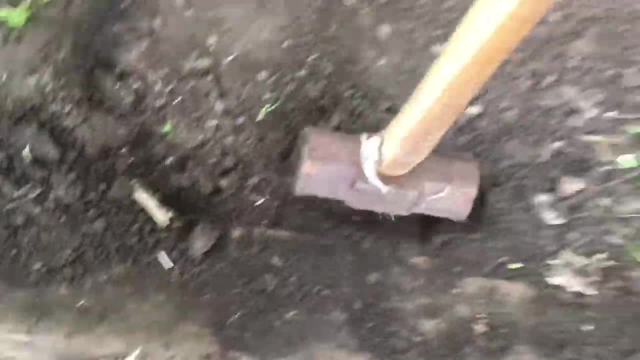 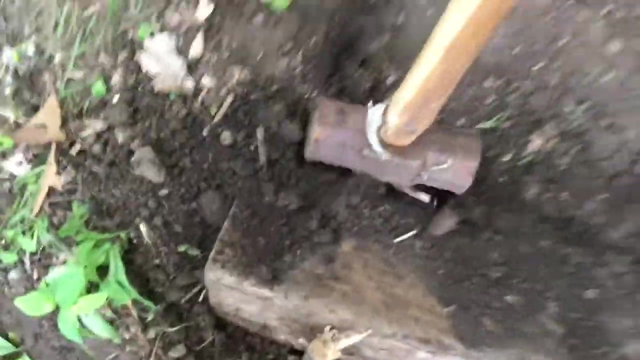 Then, once you have that in, take a sledgehammer and really pack the dirt behind the step here so that it'll push the entire step out toward the stakes. That'll really make it more solid and sturdy. Then you can add more dirt to fill it in.